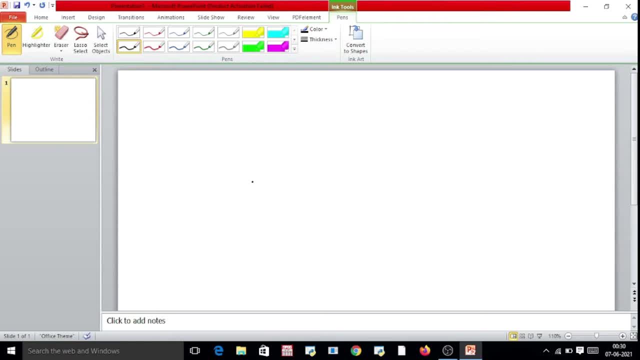 In this lecture we will learn about kernel image and their dimension. So first we see that a linear transformation, T, that maps from V to W, is defined and it is a linear transformation. Then kernel of T is defined as kernel of T, It is written as curl T, defined as a small v that belongs to the vector space V, such that T of V is equal to 0.. An image of T image is written as I. T is defined as W, a small w belonging to capital W, that is a vector space. 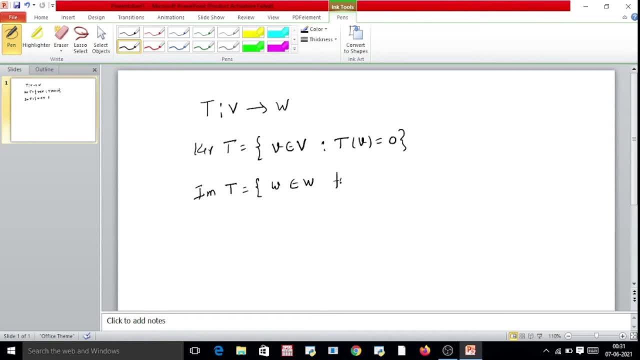 For which there exists a small v belonging to capital W, such that T of V is equal to W. The dimension of image: the dimension of image, T is the dimension of V, The rank of T and the dimension of kernel: T is the nullity of T. T, that's map from R4 to R3, be a linear transformation. 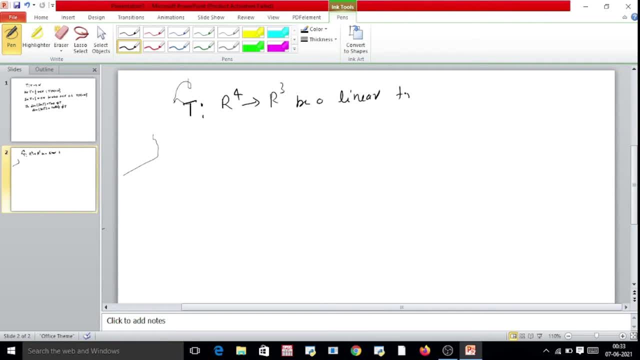 ki morph Be a linear transformation w части Defined by V. t square stays on T e x comma y comma z comma T is equal to Sy x minus y plus z plus t comma 2x minus 2y plus 3z plus 4t comma 3x minus 3y plus 4z plus 5t. 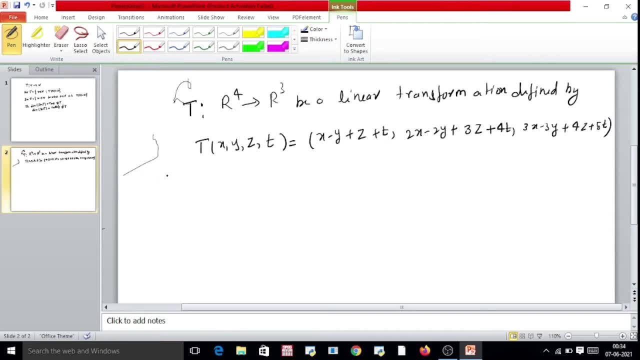 So we have to find: first, find a basis and the dimension of the image of t And second, find a basis and the dimension of the kernel t solution. So to find the image of R4.. So to find the image of R4.. 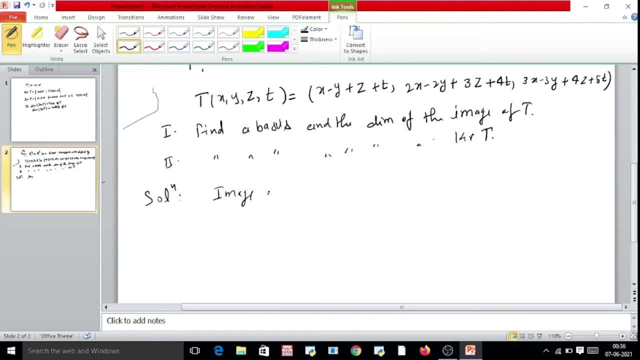 R4, first image of R4.. We proceed as follows: First write 1 comma 0 comma 0 comma 0. From here we get 1.. Then from second value here we get 2.. Then from here we get 3.. 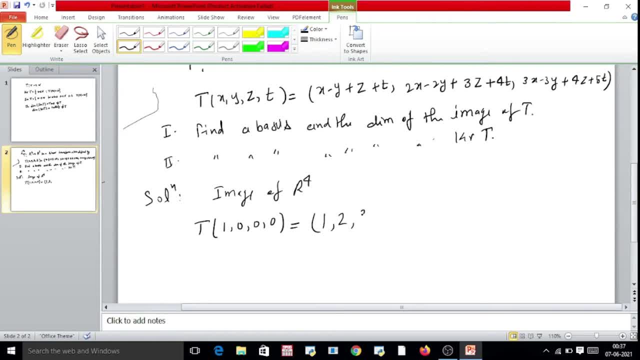 3x. if we write T 0 comma 1 comma 0 comma 0, so we get minus 1, minus 2, minus 3. we are taking all the values from here only so you may put all values and you will get what I am getting here. so T is equal to 0 comma 0 comma 0 comma 1, and this is. 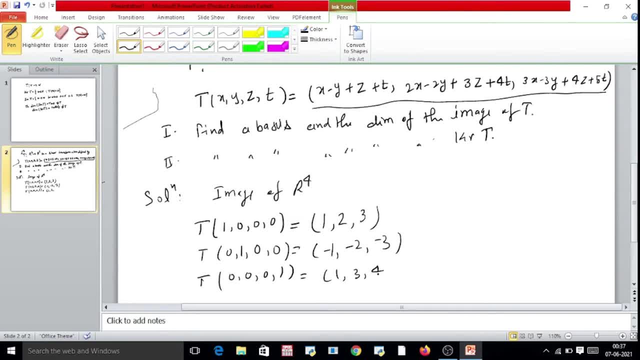 equal to 1 comma 3 comma 4, and then T is equal to 0 comma 0 comma 0 comma 1, and you will get 1 comma 4 comma 5. so now we have obtained the values and arrange them in row form. 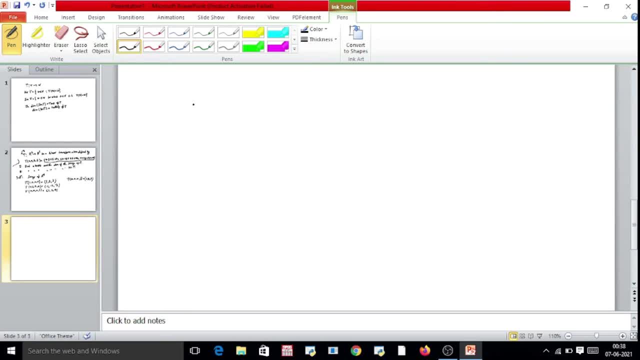 this is a matrix, so write it as: A and A is equal to 1, 2, 3 minus 1 minus 2 minus 3, 1, 3, 4 and 1 4 5. now reduce it into equivalent form. so far. doing this, we are going to take row operation, row elimination operation. 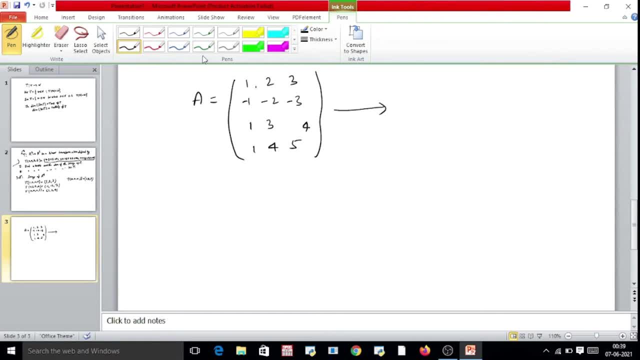 so R1 will be same, and when R1 is same, this value is pure, and below this all entries should be 0. so to make them 0, we operate like this: R2 is equal to R2 plus R1 and R3 is equal to R4 minus R1. 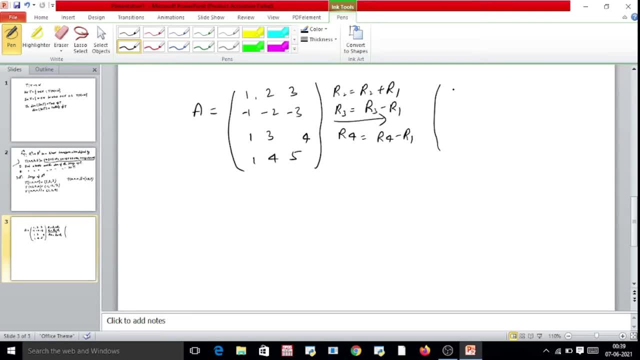 so what we get? we get one, two, three mean there is no change in first row. then we are adding first-hand row, then all of these entries would becomes 0, then R3 is equal to R3 minus 1. so see here, one minus one is zero and three minus two is. one. 4 minus three is 1, 4 minus 2 is 0 and 3 minus 2 is 1, so R3 is 1. if we apply this, we will get the increase in info, stating that that each and every times there is a. 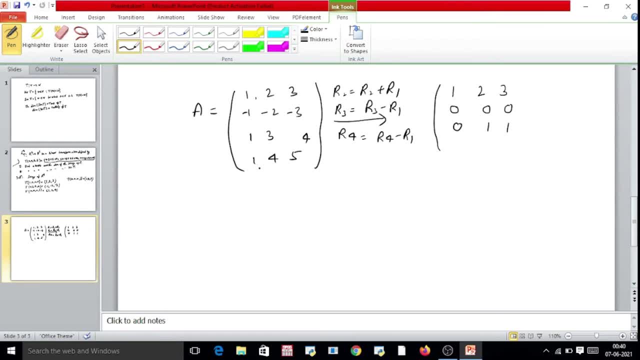 change in info, but it is not a bad thing, then unit method that we will apply is staying. then you should be able to see how we substitute, know how to write per sides. and what is вы? 1 and see: 1-1 is 0,, 4-2 is 2 and 5-3 is 2.. So again, perform row operation. R4 is equal. 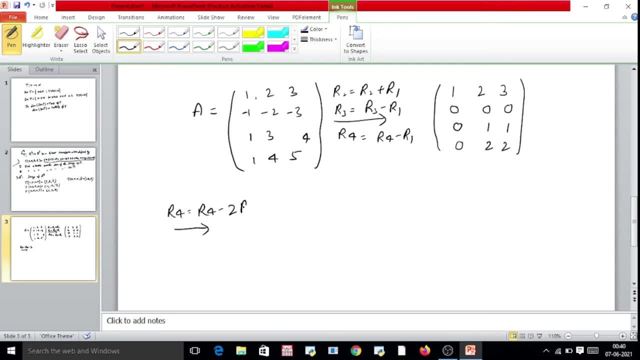 to R4-2R3.. So we will get 1,, 2,, 3,, 0,, 0,, 0, 0, 1,, 1,, 0, 0 and 0.. Now all the 0 row will. 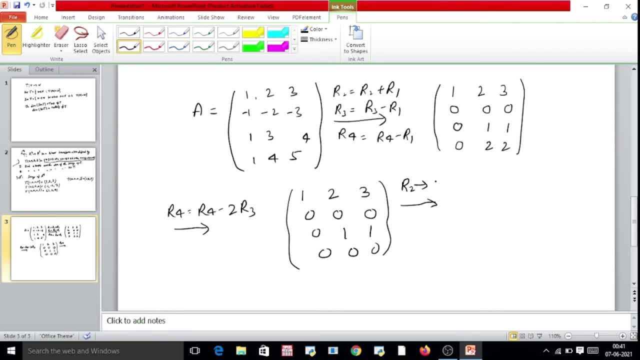 be 0. So R2 would be R3.. So this is 1, 2 and 3, 0, 1, 1, 0, 0, 0, 0, 0, 0, 0.. So. 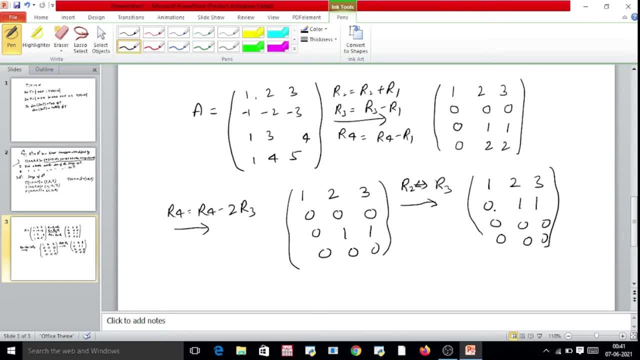 this is 1.. Here we have two non-zero rows, Two independent rows, So the rank of this matrix is 2.. So dimension of this is 2.. Since both of them are independent, so they are making the basis. So thus 1, 2,, 3,, 0, 1,. 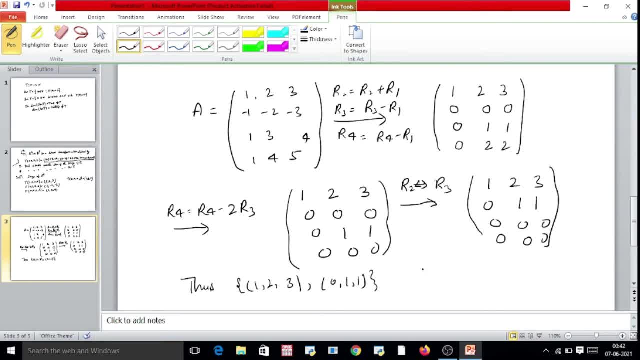 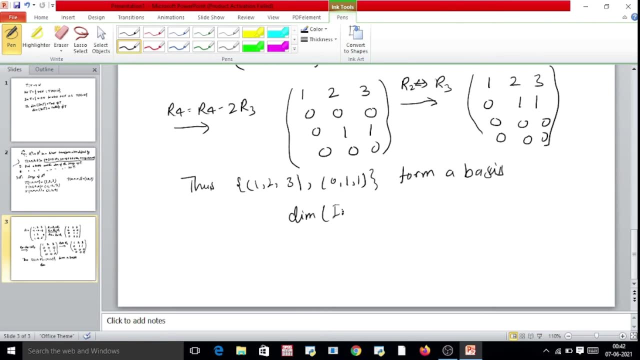 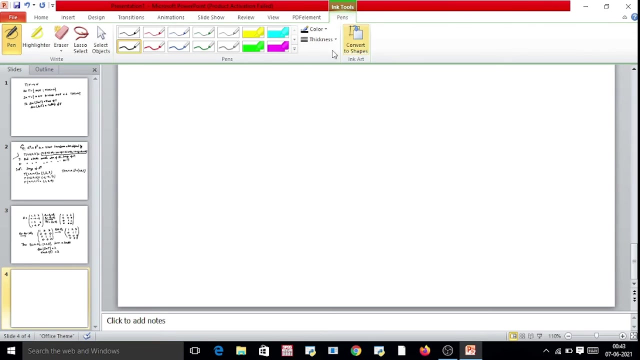 1 form a basis, Then dimension of image t is equal to 2, and this mean rank of t is equal to 2.. Now we will solve this. So we have T of t and from this we know that T of u is equal to 0.. And here it is. 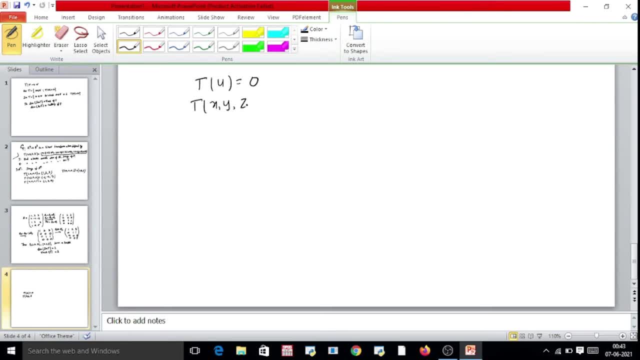 defined as T of x comma y comma, z comma t is equal to x plus y plus z plus t, comma 2x minus 2y plus 3z plus 4t comma 2x comma 3x minus 3y plus 4z plus 5t, and this is equal to 0 comma 0 comma, 0 comma 0. so from here, 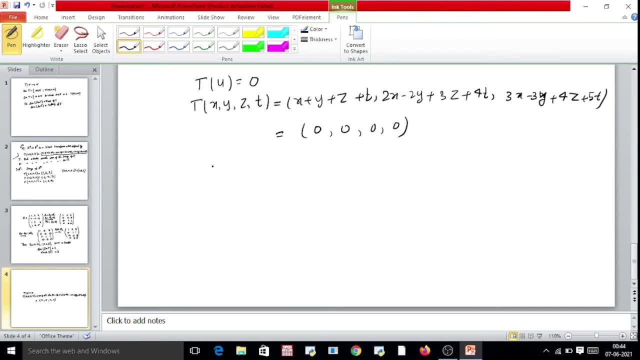 we obtain a matrix, we obtain this system: z plus t is equal to 0, and then 2x minus 2y plus 3z plus 4t is equal to 0, and then 3x minus 3y plus 4z plus 5t is equal to 0. 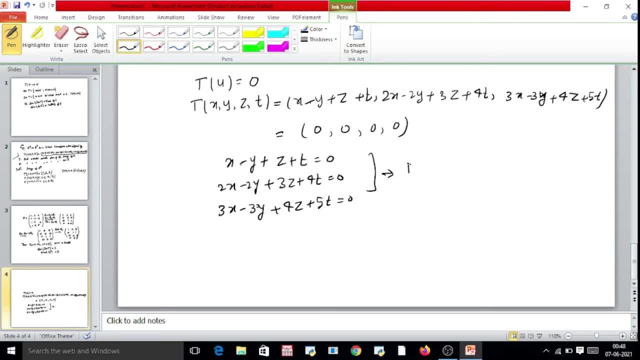 so from here we find a matrix m and it is as: 1 minus 1, 1, 1, 2 minus 2, 3 and 4, 3 minus 3, 4 and 5. now again, we want to reduce this form, this into echelon form. so this is first. 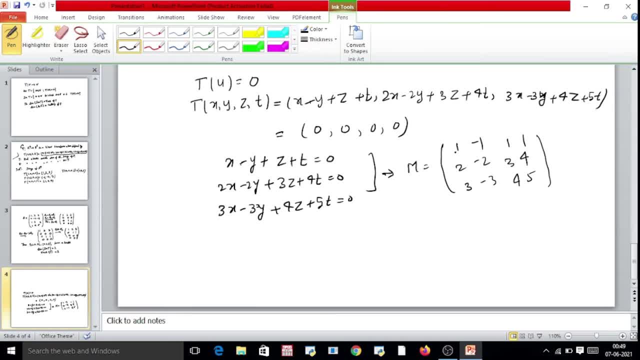 would be same. this is 1 And this is pivotal element. Sorry, below the pivotal element, all entries must be 0. So to make them 0, we proceed as follows. We are going to operate unrow, So R2 is equal to R2 minus 2R1 and R3 is equal to R3 minus 3R1. 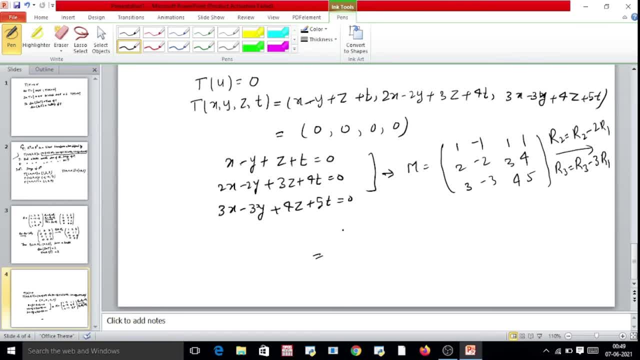 So from there we get 1 minus 1, 1, 1, and this is 0.. 2 minus 2 is 0.. Minus 2 and plus 2 is 0.. 3 minus 2 is 1.. 4 minus 2 is 2.. And then for row 3, 3 minus 3 is 0.. Minus 3 and plus 3 is 0.. 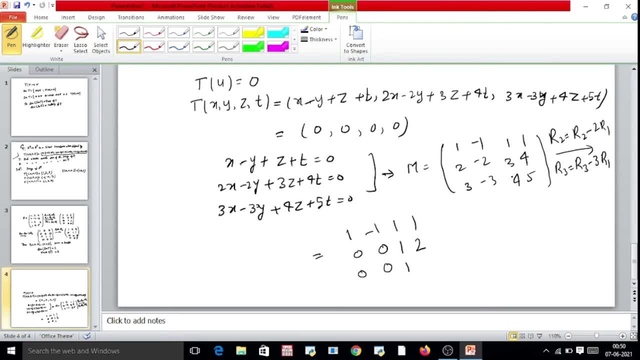 4 minus 3 is 1 and 5 minus 3 is 2.. Now again apply operation unrow, So R3 is equal to R3 minus R2, and what we get? 1 minus 1, 1, 1, 0, 0, 1, 2, 0, 0, 0. 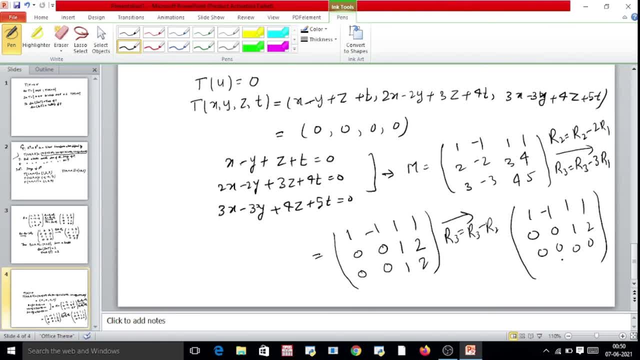 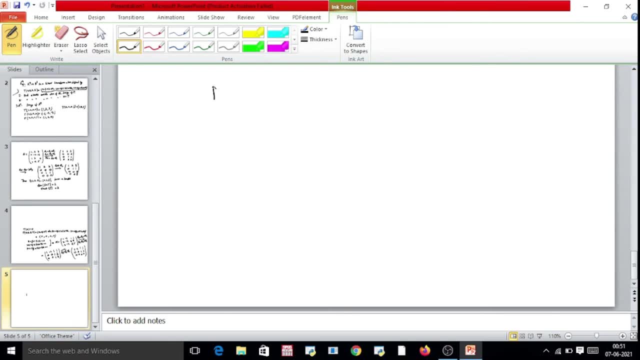 0 and 0. So from here we have 2 independent variables among 4.. So from above, mx is equal to 0.. And m, reduced form of m, is 1, minus 1,, 1 and 1.. 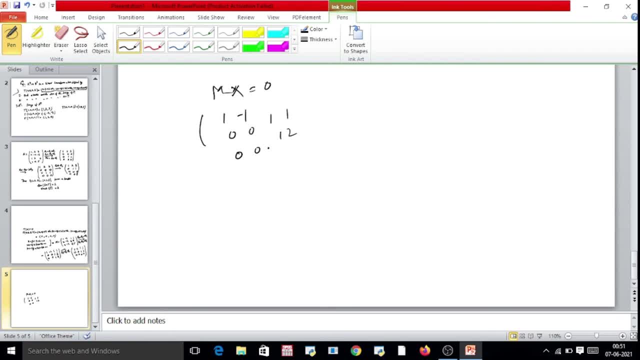 0, 0, 1, 2, and then 0, 0,, 0, 0.. And x is x1.. y, z and t is equal to 0.. So from here we get 2 equations: x minus y plus z plus t is equal to 0. 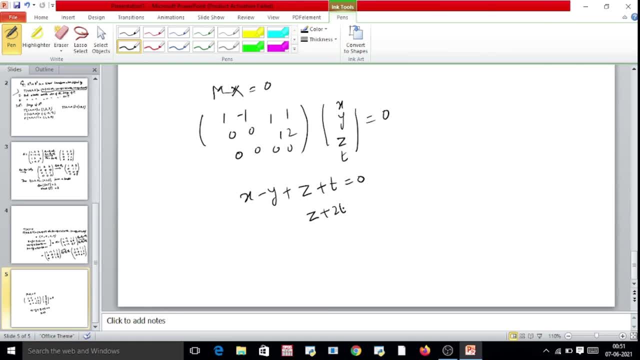 And z plus 2t is equal to 0.. See, here we suppose, that here 2 variables are free. Here 2 variables are free. Which variables? y and t are free. See how. So z is equal to minus 2t and x is equal to y. sorry, x minus y minus 2t plus t is equal to 0. 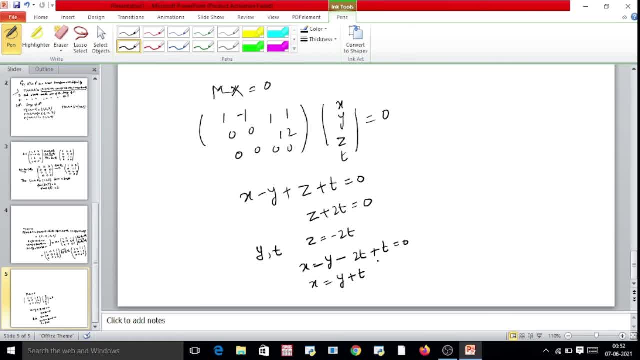 So x is equal to y plus t. So from if we take sorry, y and t are free, we may take any value of them. So just suppose t is equal to k1 and y is equal to k2, then what we get, z is equal to. 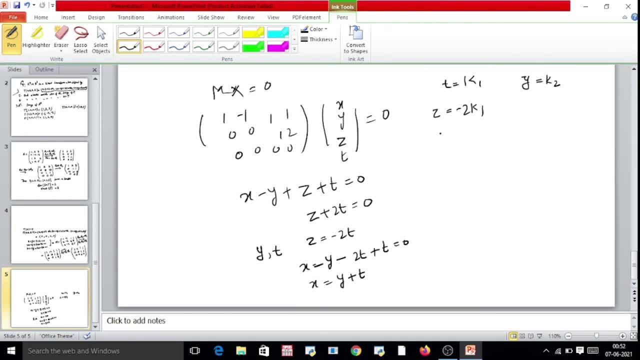 minus 2k1 and x is equal to k2 plus k1.. So from there we get: x, y, z and t is equal to k1 plus k2, then k2, then minus 2k2.. So from there we get: x, y, z and t is equal to k1 plus k2, then k2, then minus 2k2..